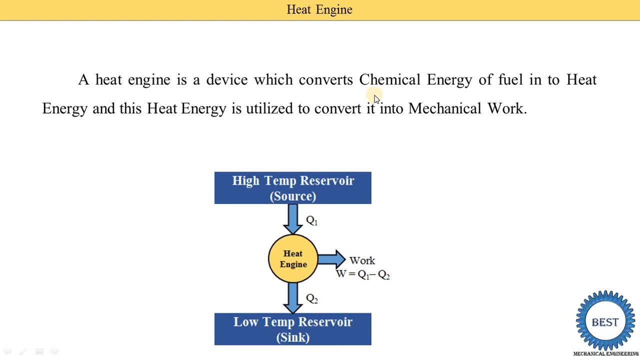 So in bike we fill the petrol. So in a petrol there is a chemical energy. So when we supply this petrol in IC engine it is converted into the heat Means. the chemical is converted into the heat and then, after this heat energy and this heat, 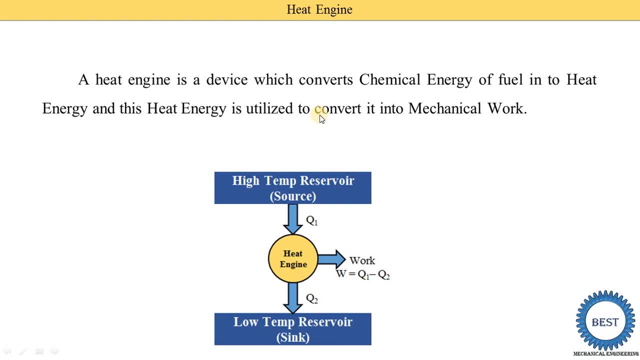 energy is utilized to convert into the mechanical work. Suppose we talk about the nuclear power plants. So nuclear power plant, we use the uraniums or a platinum as the chemical source and in this nuclear various reaction is there, that is, a fission. fission reaction is occurs on that nuclear and they release the heat energy. 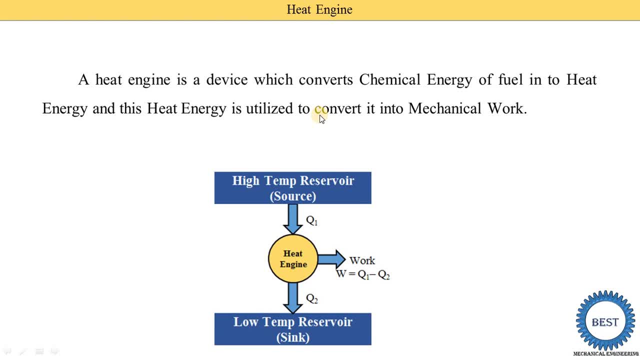 So here is the process of loving this thermal energy and this heat energy, absorbed by the waters or some under هذا medium, and then it is supplied to the turbine, and turbine produce mechanical work means, that is, the various examples of the heat engine that is. 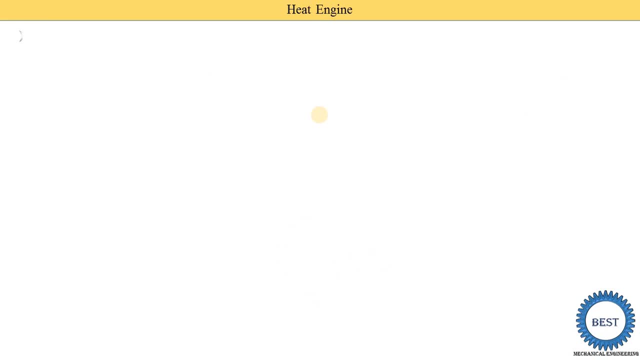 a petrol engine, diesel engine, Rankine cycles, Breton cycle, nuclear power plants are the examples of the heat engine. It is a thermodynamic system operating in a cycle. Okay, so here we need to focus on the час, FPS. That is the cycle, Because here we have an insane machine that can 가 credito: surger favorece an Water eldo sifál o sommer morte. 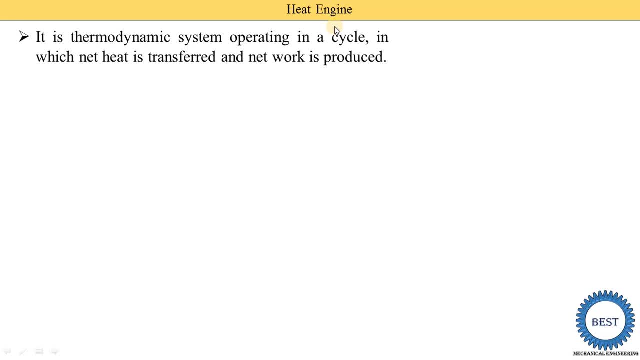 cycle means in a cycle there is a number of processes that okay. no single components make the heat engines okay. so in a heat engine, number of process is there means more than one process is that in which net heat is transfer and net work is produced. so when we use the net heat and net work, that means in a 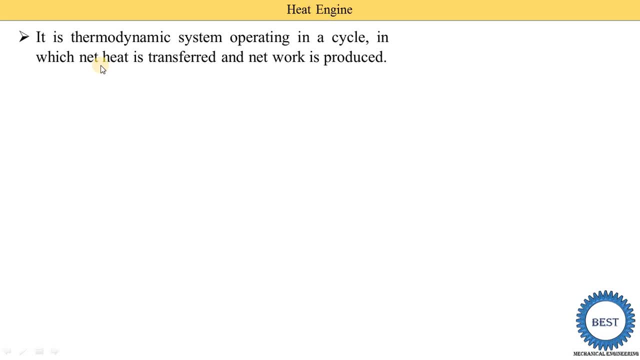 more than one component that is a heat interaction is going on and network word is used, that means more than one component in which the work interaction is going on. here I use the work interactions and heat interaction work because in heat and work it is possible that either we supplied the heat or we. 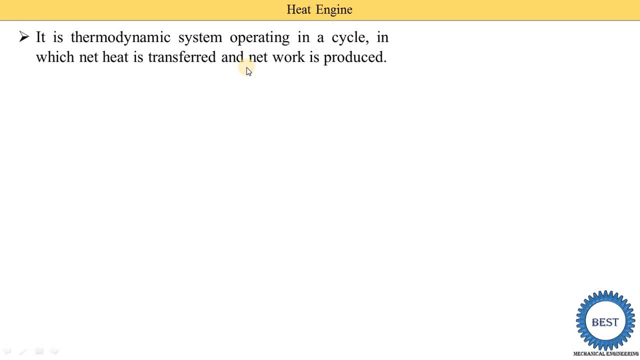 reject the heat. either we supplied the work or either the work is produced by the systems. heat engine is a work producing device, as shown in this figure. so every device that have the two type, either to work producing device or a work consuming device, but the heat engine is a work producing device, as shown in this figure. so every device that have the two type, either to work producing device or a work consuming device, but the heat 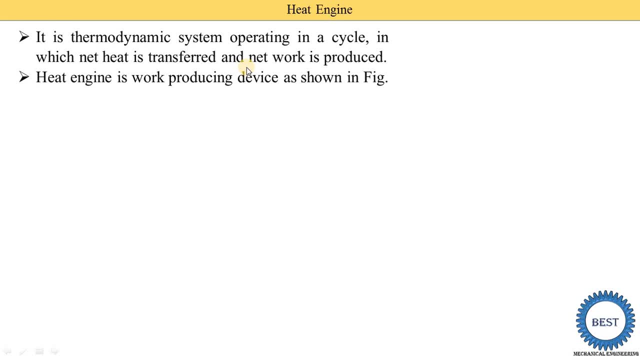 engine is a work producing device. okay, that means we supplied the heat energy and it's produce some mechanical work. now, in this component that is a major part is that source is that sink is there and heat engine is there. okay, so here you see. this is the high temperature reservoirs, so it is called. 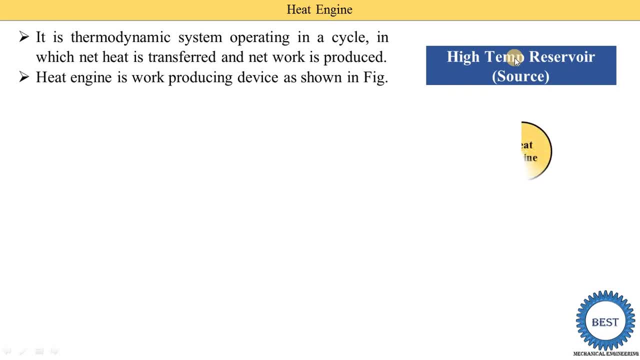 as the source, from the source we supplied the heat energy to the heat engine. okay, so here you see, it is the downward arrow and it is towards the heat engine. that means we supplied the heat energy to the heat engine and quantity of the heat energy is the. 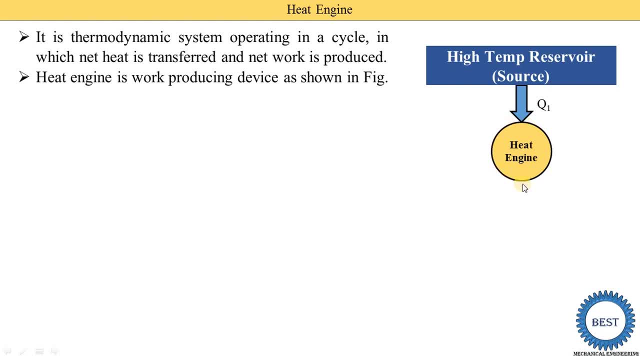 q1, okay, and this heat engine is convert heat energy into mechanical, but that means they produce mechanical work. that means we draw this outward arrow, that means the output is coming from the heat engine and it is the work. an equation of the work is: q1 minus q2 means we supplied the q1 and this heat engine is. 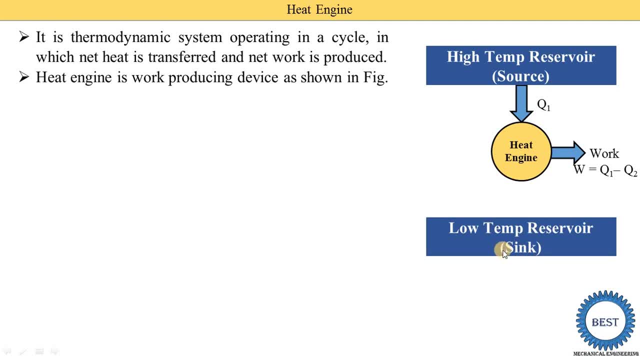 reject the q2 quantity of the heat to the sink. okay, so here the low temperature temperature reservoir and it is called as the sink. so in a sink the heat engine is: reject the q2 quantity of the heat. energy means how amount of the work is produced. the work produced is the 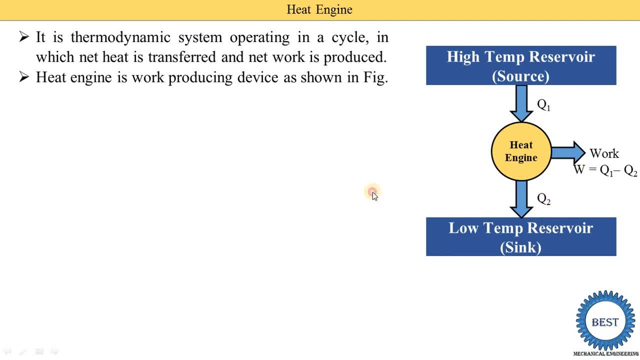 heat supply minus heat reject. so it is used to produce maximum work for a given positive heat transfers. the characteristic of heat engine as followed: first it receive a heat from high temperature source. so here in this diagram you see, here heat engine is there and this is the. 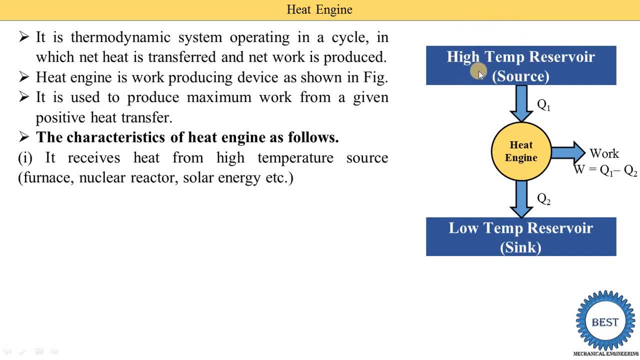 high temperature reservoir. okay, so as a high temperature reservoirs we can use the different component, that is, a furnace, nuclear reactor, solar energy- okay, so that we already discussed. suppose that is a steam power plant, is there? okay, so here the high temperature reservoir is that is a boiler. 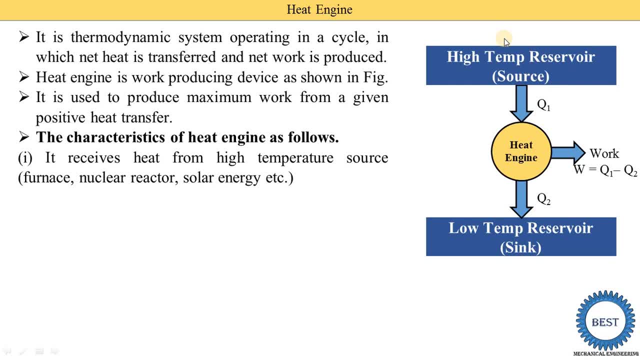 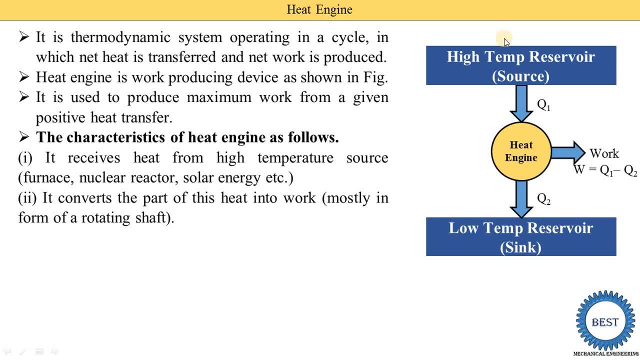 heat into work, mostly in a form of the rotating shaft, means this heat engine is convert this heat energy into mechanical energy, and this output is generally in a terms of rotations of shaft. third, it reject the remaining waste heat to a low temperature sink. low temperature sink: here you see that the heat 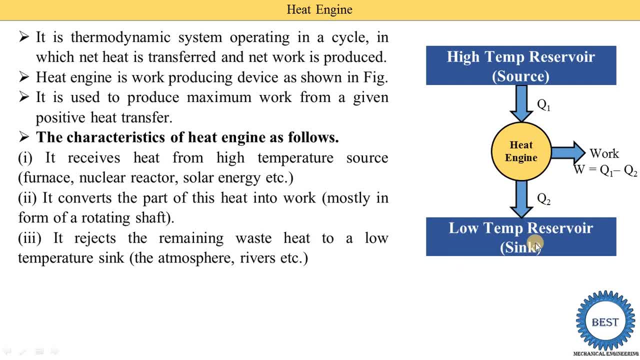 engine is reject due to quantity of heat, to the sink. and in actual, the sink means it is a atmosphere or it is a river, means: suppose the water is coming, then water is supplied to the rivers. suppose some gas is coming, then gas is supplied to the atmospheres and, fourth, it operate. 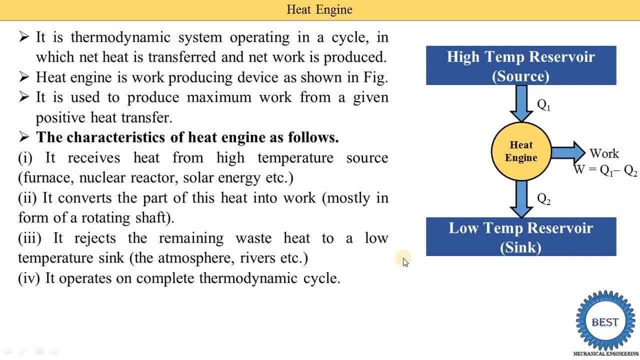 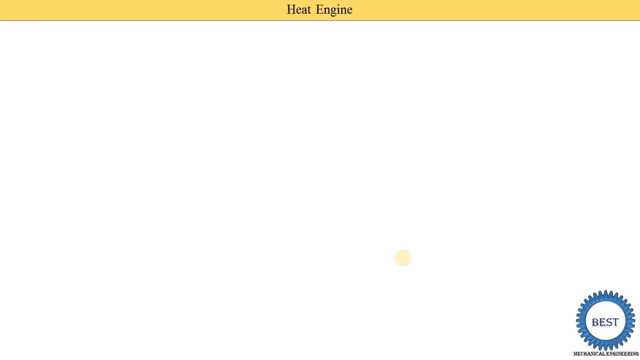 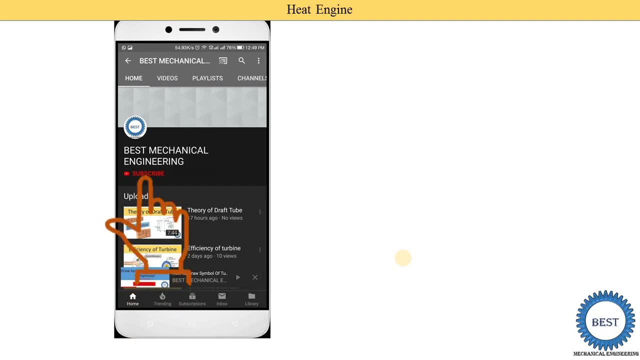 on complete thermodynamic cycle. how to complete thermodynamic cycle means in a cycle that is, a number of process is there. before moving ahead, i request to like my video and subscribe my channels for watching the more video related to engineering, thermodynamics or a basic mechanical engineering. 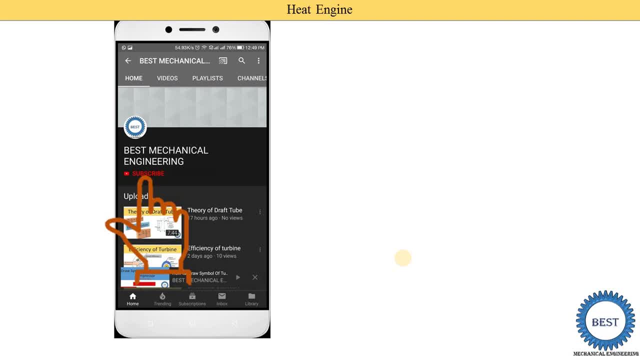 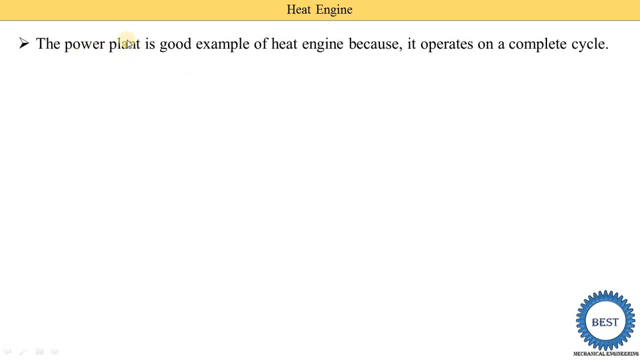 or other subject of mechanical engineering. for the engineering thermodynamic subject, various link is provided in descriptions as well as in a car. for other subject, i request to visit the playlist. now we take the one examples of the heat engine, okay, and the example we take is related to the power plant. the power plant is a good examples of heat. 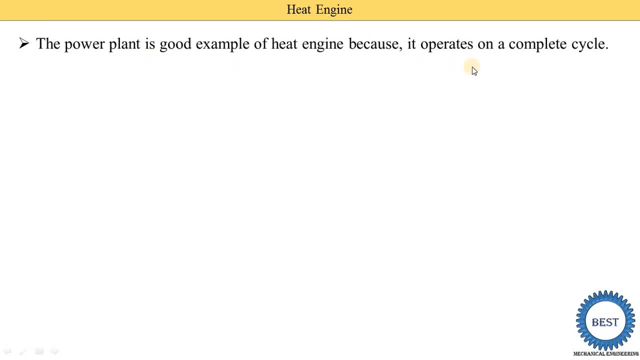 engine because it operate on a complete cycles. so here you see, this is the examples of the steam power plants. okay, so in a steam power plant, boiler is there? okay, in a boiler we supplied the heat energy. so here heat source is mentioned and it is a furnace. 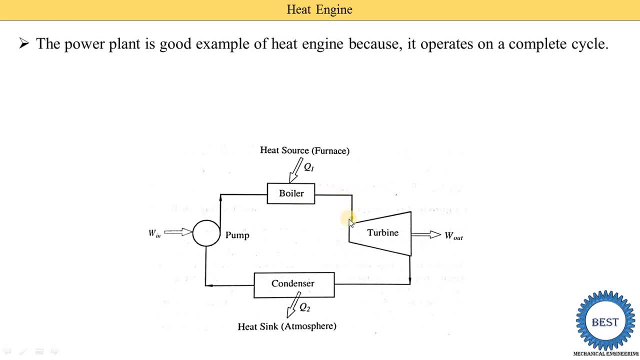 so here we supplied q1 quantity. then after steam is supplied to the boiler, in a boiler the steam is expand and some work is produced. here you see outward error, that is a work outputs. and then, after the steam is supply in condenser, in a condenser the steam is converted. 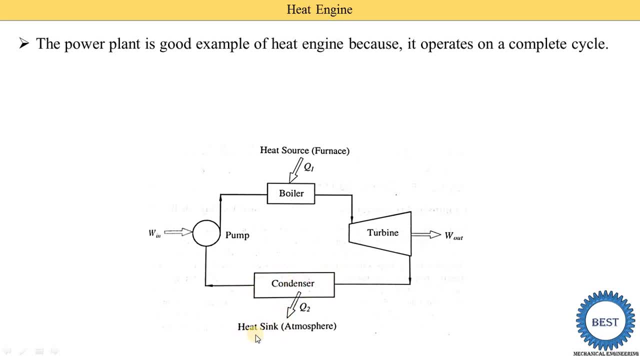 into the liquid by rejecting the heat to the sink. here you see, heat sink and it is the atmospheres. and then after water is supplied to the pump, in a pump we supply some work dance. and then after water is supplied to the boilers, means. here you see, that is a two. 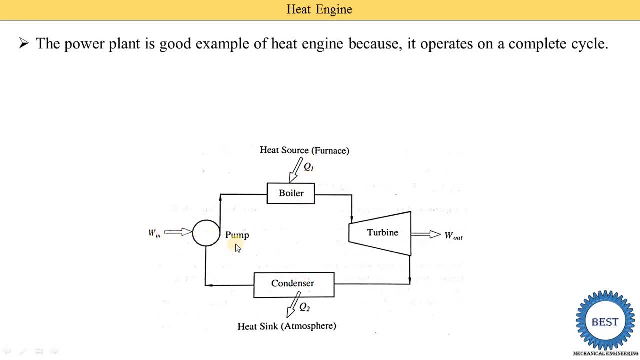 heat interaction is going on, that is a q1 and q2 and two work interaction is there, that is w in and w out. but boiler, condenser, turbine, pump separately, not heat engine, because each does not complete a cycles means we not. we cannot say that the boiler is heat engine, we cannot say turbine is heat engine. 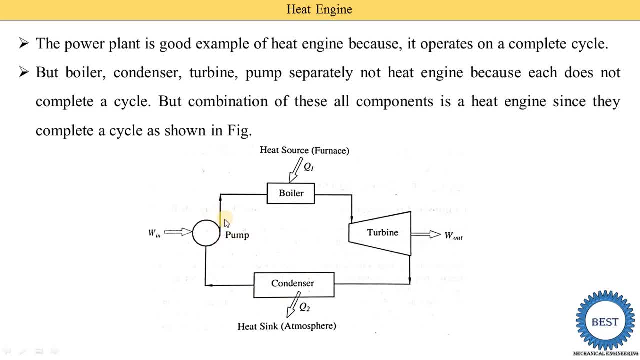 we cannot say condenser is heat engine. we cannot say the pump is heat engines, okay, because they are not complete the cycles, but combination of these all the component is a heat engine since they complete a cycle, as shown in this. figures means we consider these all. the four component is combined. at that time it's make the 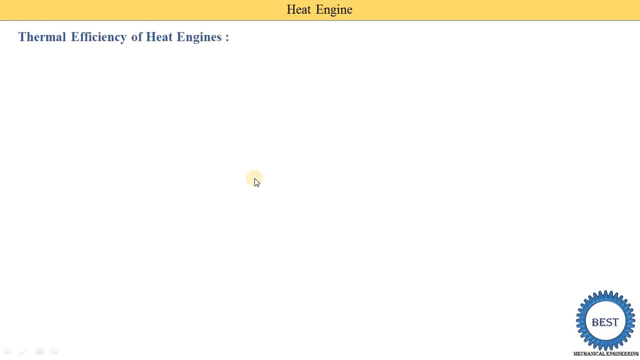 heat engine. now we find out the thermal efficiency of heat engine. so first we study what is the equations of efficiency or a definitions of efficiency. thermal efficiency of heat engine is the ratio of network output to the energy input means. in any component efficiency means it is the output of an input. so in a heat engine outward, 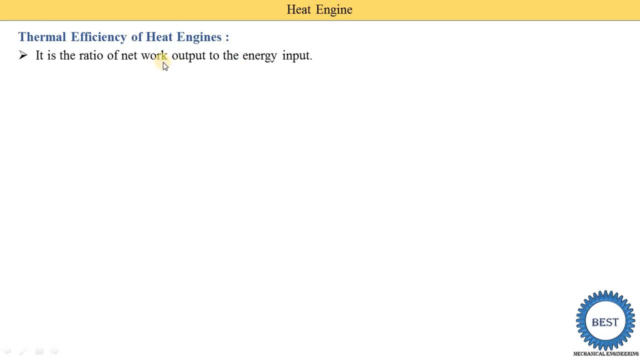 is in the form of work, so that here mentioned the work outputs, okay, and energy input. so we know that the energy input is in the form of heat energy. so again, we use this diagram for our derivations. so only fraction of heat input is converted into the work and demand heat is rejected. so we know. 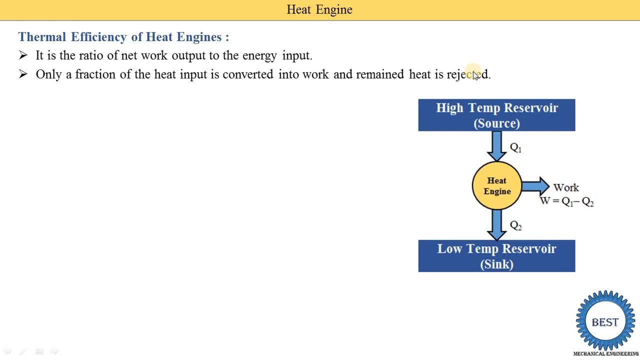 that the heat is the low-grade energy and it is not completely converted into the work. okay means efficiency is never more than 100 percent. it is always less than to the 100 percent okay. so here you see that the v supplied the some q1 quantity of heat and out of this q1, some quantity of the. 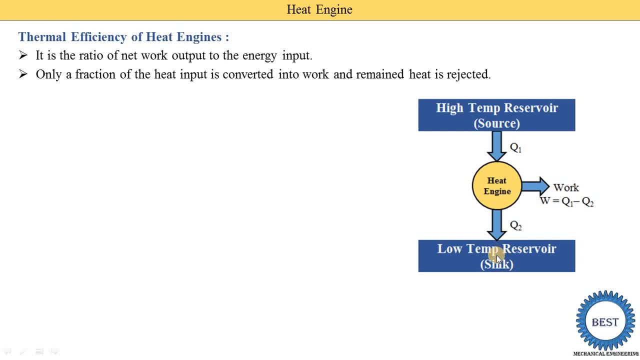 heat energy is converted into the work and some quantity of the heat is rejected to the sink. okay means the efficiency is on a fraction of form. so here we consider that q1 is equal to heat supplied to the system, and unit is the kilojoule. 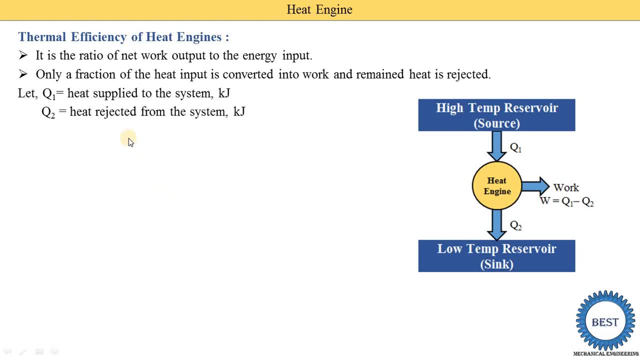 so here we consider that q1 is equal to heat supplied to the system and unit is the kilojoule, Second, Q2.. Q2 means heat rejected from the systems in a kilojoules. So here you see this Q2, it is called as the heat rejections. and here you see, this is the Q1, it is called. 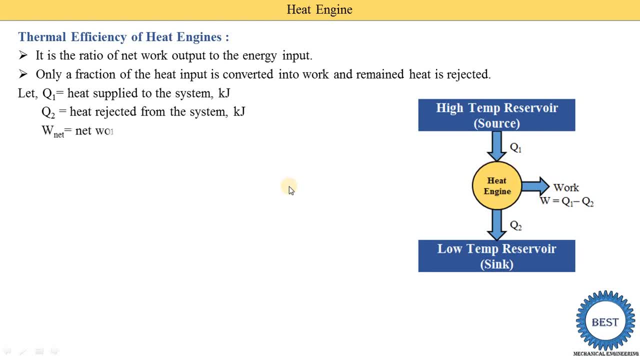 as the heat supplied to the heat engine And Wnat nat work done by the system in kilojoule. So here that is, Q1 minus Q2 is equal to the work, or we also say that it is the nat work. 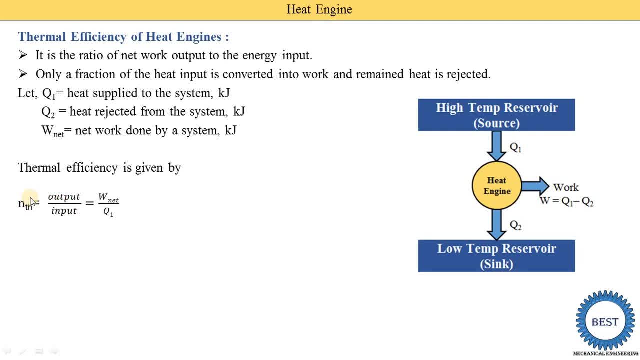 Thermal efficiency is given by this equation: efficiency, thermal is equal to output upon input. So output is the nat work done and input is the this Q1, heat energy. So we return this equation: Wnat upon Q1.. So our output is the work, And here we also able to return. 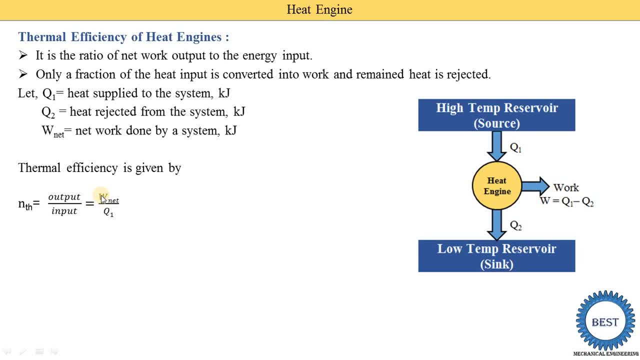 this work. but in a heat engine there is a number of component. Okay, earlier we see that is the pump and turbine is there, Turbine is produce the work and the pump is consumed the work. we need to mention the w networks and input is only one, that is a heat input, that is the q1. 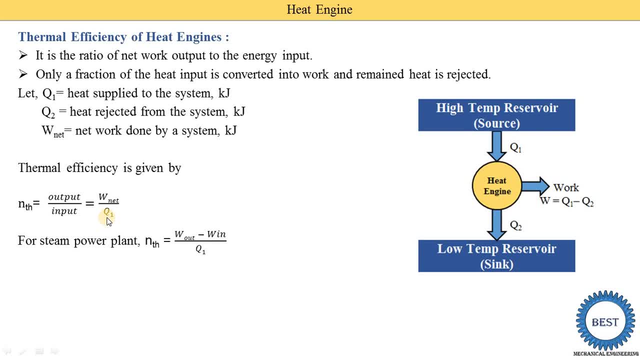 now for steam power plants. the thermal efficiency is equal to w out minus w in divided by q1. that why already explained, that is, a turbine work is in output and the pump work is the input. now we know that the first law of thermodynamics. okay, what the first law of thermodynamics say? 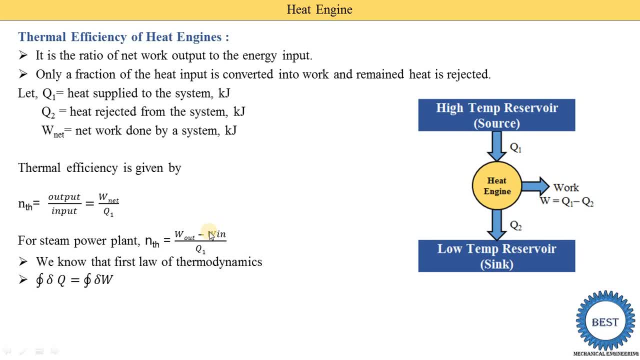 that cyclic integrations of heat energy is equal to cyclic integrations of work energy. okay, so in a steam power plant we see that that is a two. two heat interaction is doing that, one in boiler and one in condensers. okay, so here we mentioned that is a q1 minus q2, because one is 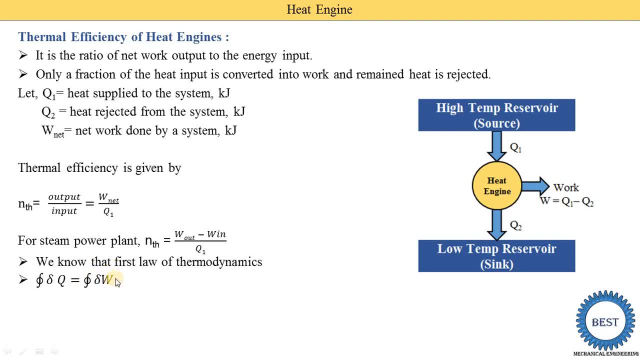 supply and one is reject and work interaction, that is, a turbine work minus pump work. so here we consider that the cyclic integrations of heat energy is equal to w out minus w in, divided by q1 minus q2, according to these diagrams. okay, and work integration is the w net. now we putting this: 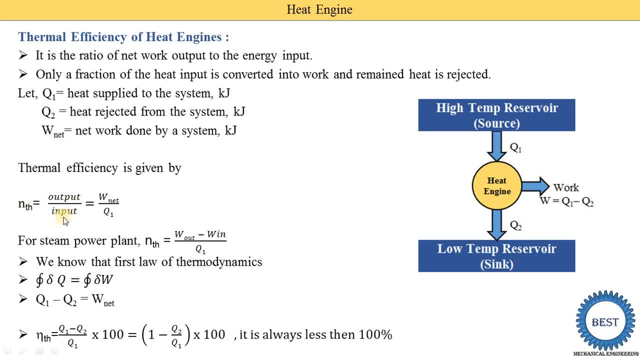 value in these equations. okay, so this equation here you see this w net. okay, so what is the equation of w net? it is the q1 minus q2. okay, because of these equations, okay, here, the we know that the w net is in term of the w, that is, the w out minus w in. but according to this first,